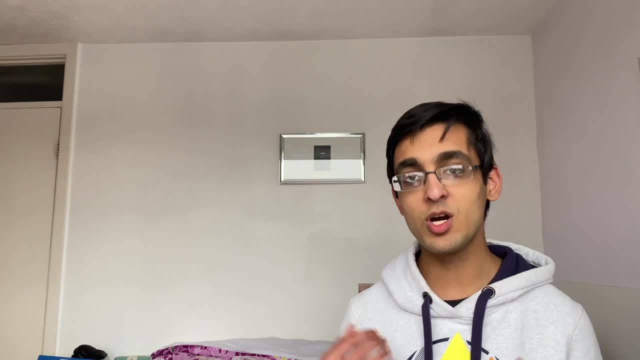 had names in and link across the entries and de-anonymize people. Strava also found out that just removing names doesn't preserve privacy of the data, So when they released an anonymized aggregate heat map of location data from across the world, it found that they actually released sensitive. 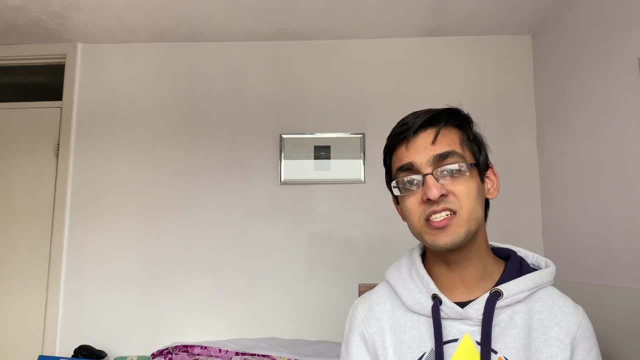 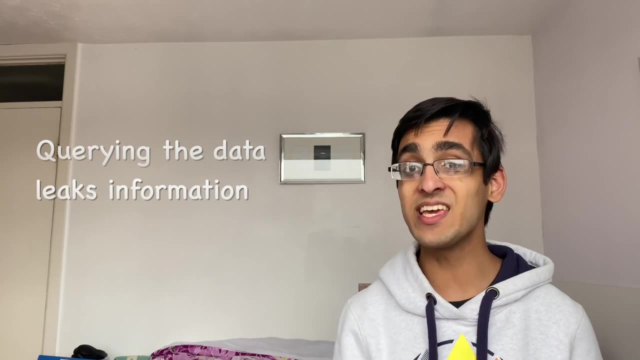 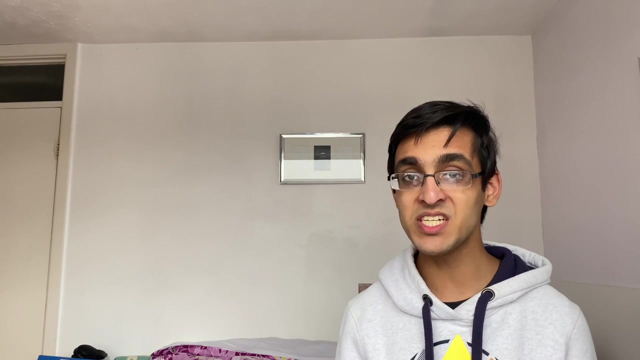 data about military locations. It turns out that every time we query a data set or form some sort of statistical analysis, we're leaking information about the data set. Saying that we don't want to learn anything about the data set and have total privacy is unworkable. Instead, we want: 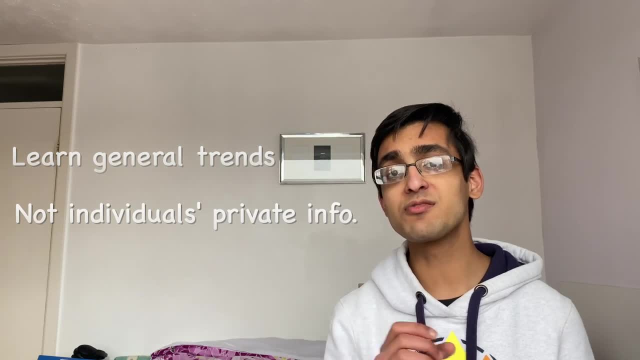 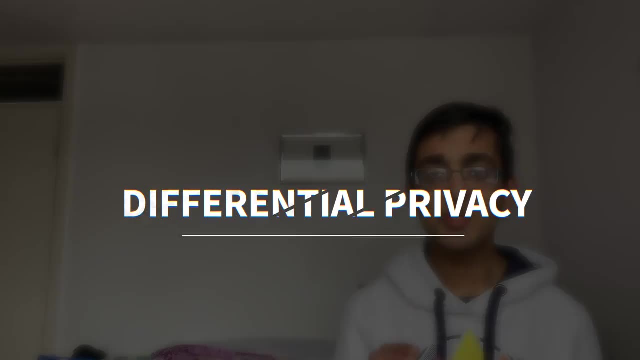 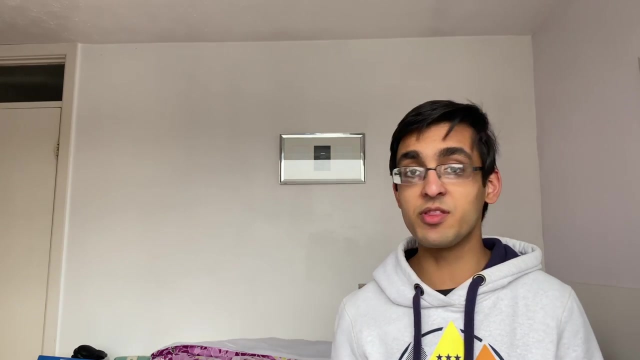 an ocean of learning from the general trends of the data set without revealing individuals private information, And this is the key idea behind differential privacy. Differential privacy analyzes the privacy of any mechanism that accesses the data and produces some sort of output. So this could be your database queries, It could be a pen and paper query And in our case, it's the entire. 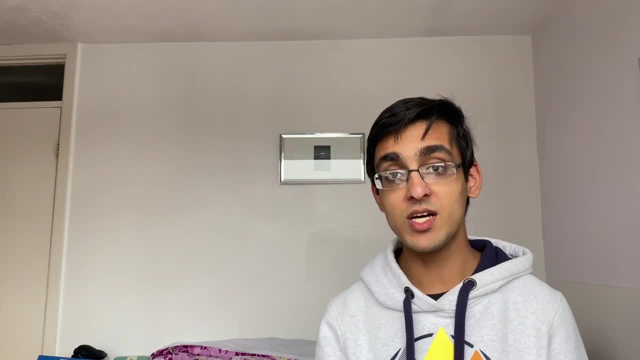 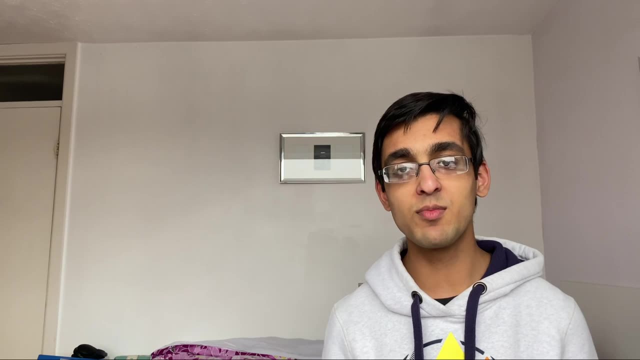 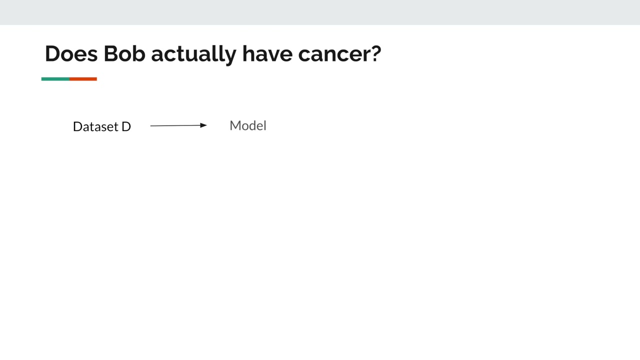 process of querying the data to train our model and then using our model for predictions, Not just the final model, that entire process. Say, we're training a model on a medical data set D, and we want to predict whether a particular patient, Bob, has cancer or not, And this model that's. 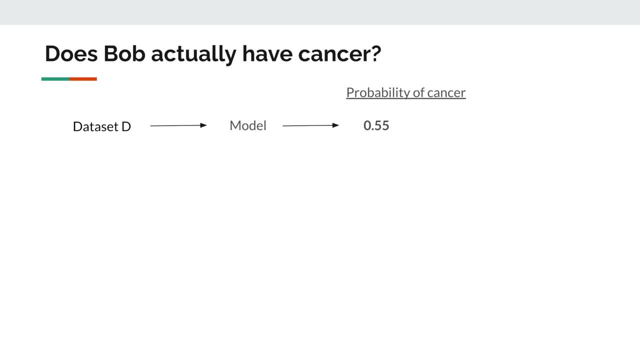 been trained, comes back and says it has a 55% confidence That Bob does have cancer. Now say we took the same model but trained it on the same data set plus Bob's data, And it comes back and says that actually I have a 57% confidence that Bob has. 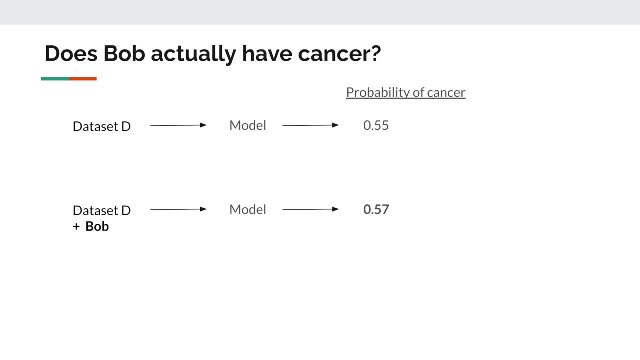 cancer. This doesn't necessarily mean that Bob has cancer, right, Because Bob could just say that, oh, it's just because the machine learning model had more data So it was able to form better and be more confident in its predictions. So he has this plausible deniability, And that's the key to 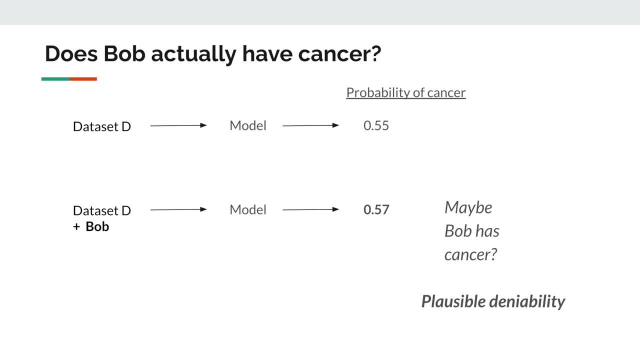 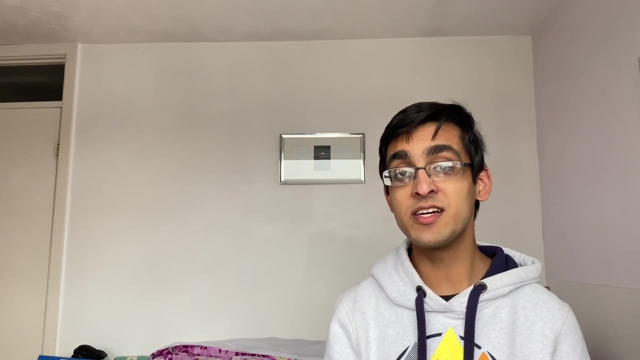 privacy. However, if the machine learning model had predicted 80% after we'd added Bob's data, then it's pretty clear that Bob does actually have cancer And the prediction of the machine learning model has actually leaked information about Bob. The key thing to note here is that we're leaking. 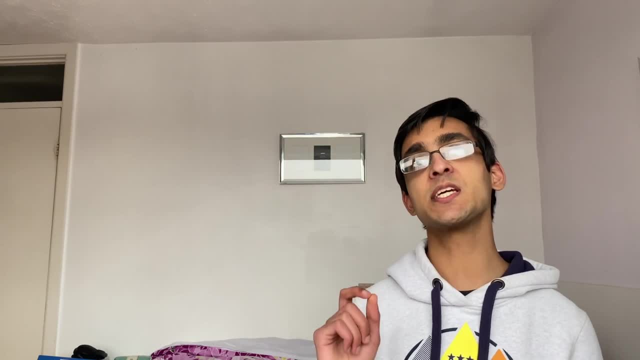 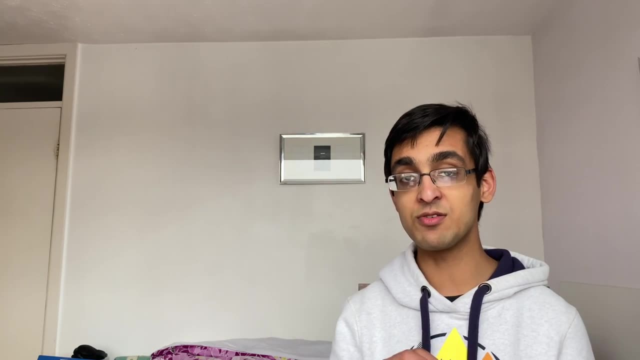 information about a particular data record. Every time a particular outcome becomes suddenly much more likely or unlikely after we've removed or added that data record from the data set. And we can quantify this by looking at the log of the ratios of the two probabilities. So the log of 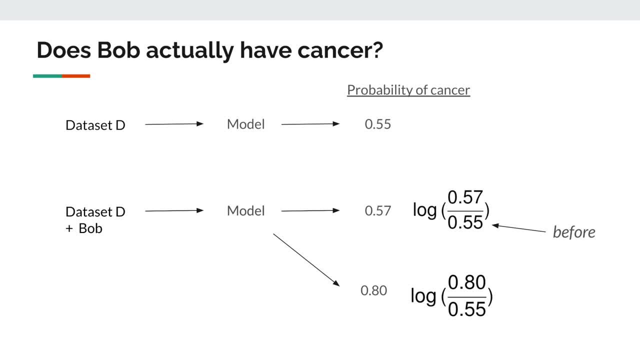 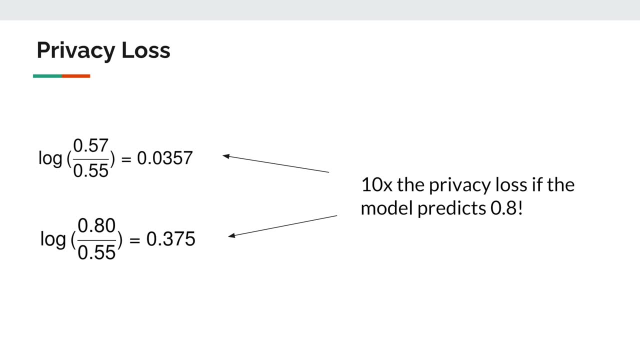 the ratio of the probability before we'd added Bob's data to the data set and after, And so we can quantify this as the privacy loss when training on Bob's data. The key idea behind differential privacy is that we want to limit this privacy loss for a particular individual. The model: 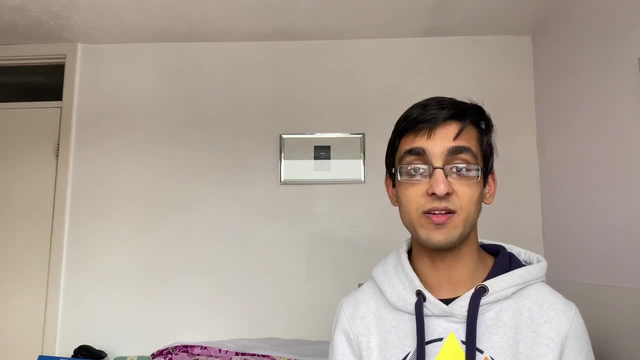 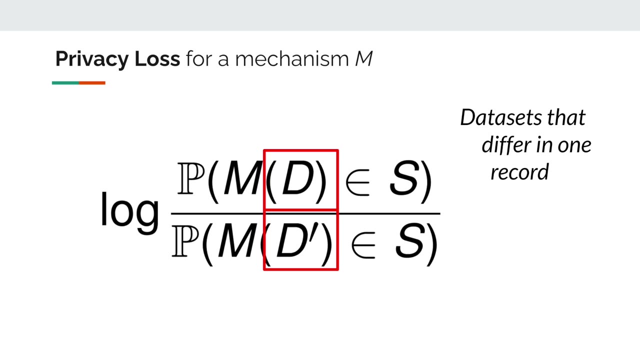 should make a similar prediction about me, whether or not I opt into the data set. So in general, we look at data sets D and D prime that differ only in one particular data record And we look at the probability for a set of outcomes, S, And we can bound this log probability by Epsilon. 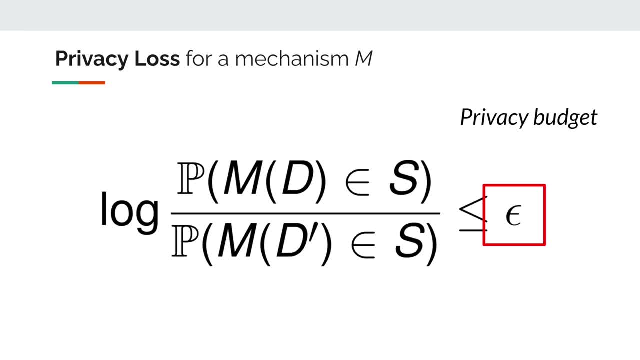 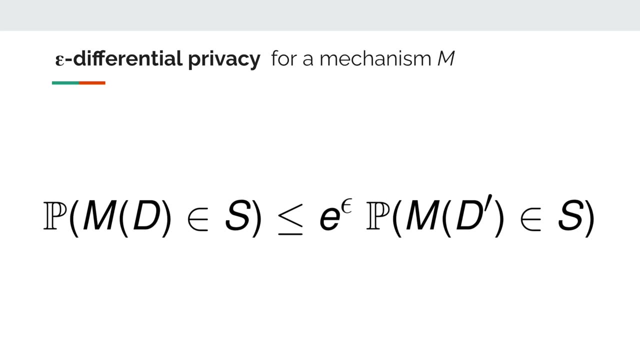 which we're going to call our privacy budget, And so, obviously, zero privacy loss is great, but you're going to get the same probability before and after until you've learned nothing, And so we can tune this Epsilon to trade off between privacy and learning about the data. We can rearrange this inequality, And this is the 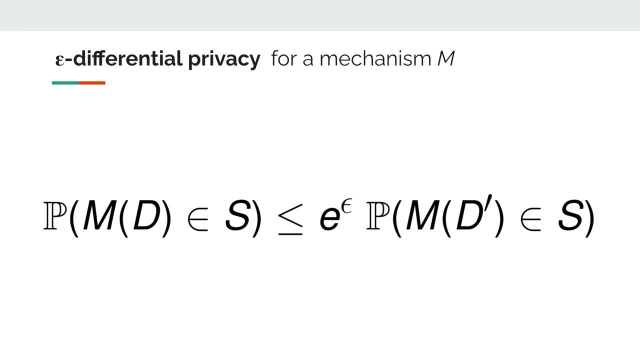 more traditional definition of differential privacy. Now if we can show that this inequality holds for all data sets D and D prime and for any set of outcomes S, then we say that our mechanism M is Epsilon differentially private And this guarantee is pretty strong. So in practice, 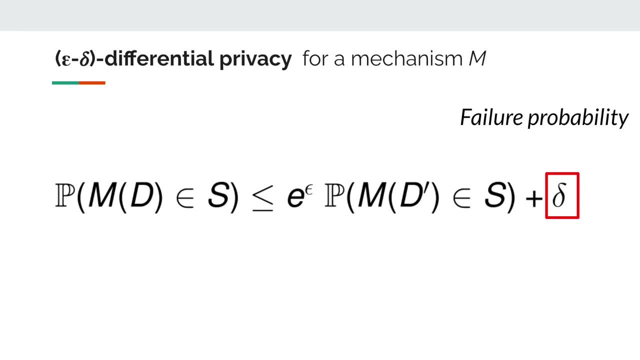 we actually define Epsilon Delta differentially private. where Delta is a failure probability And so long as this probability is much less than any particular individual's probability, this won't affect the privacy in practice, but it allows us to prove the balance much more easily. So I want to take a moment here to pause and just reflect on how. 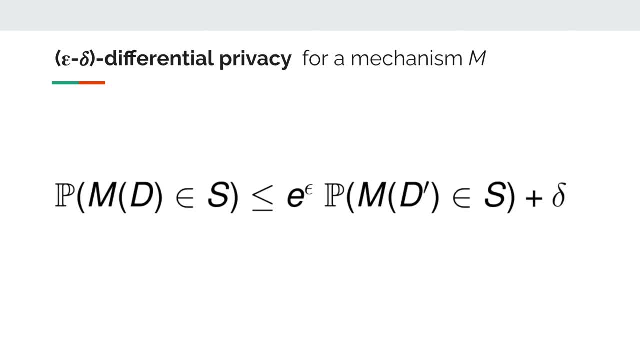 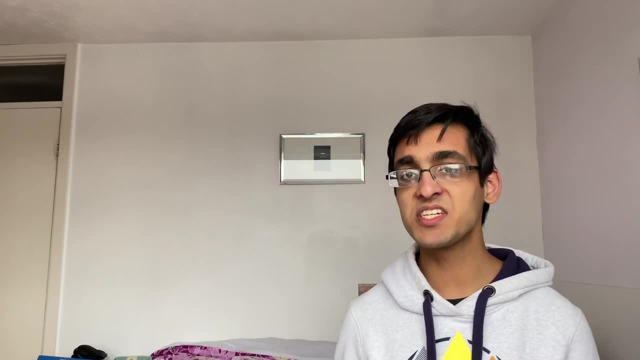 elegant. the solution is: No longer is privacy subjective. We can actually compare quantitatively the Epsilon Delta values for different algorithms And this privacy guarantee is rock solid, no matter how the attacker decides to post-process our data or to combine it with other auxiliary data. 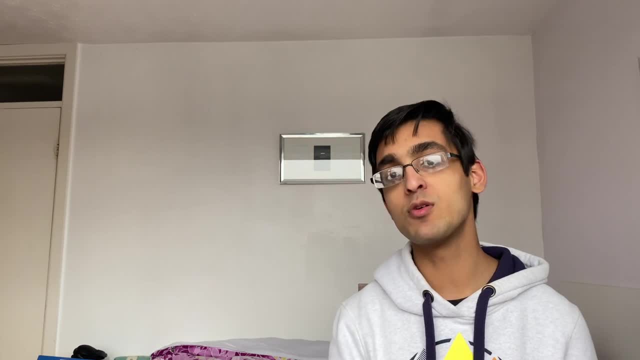 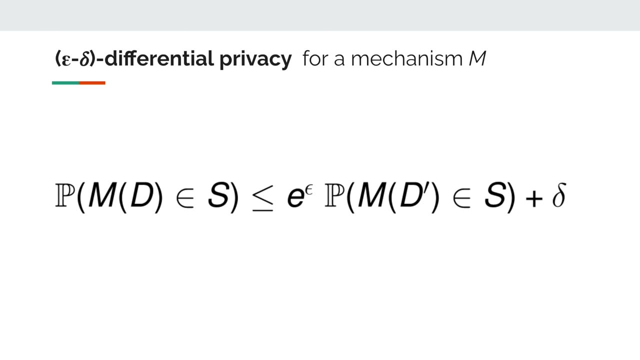 and link it. we know that we're not going to be leaking any more information than this bound that we've given. So now that we have this definition of differential privacy that has these formal guarantees, how do we actually achieve it? We can limit privacy loss by adding noise to our output. So think of an image. The more blurry the image, the less you can tell. The more noise we add, the smoother the range of possible outcomes, And so no one outcome is that much more likely than the other. And the smaller our privacy budget, the more noise we have to add to smooth over more. 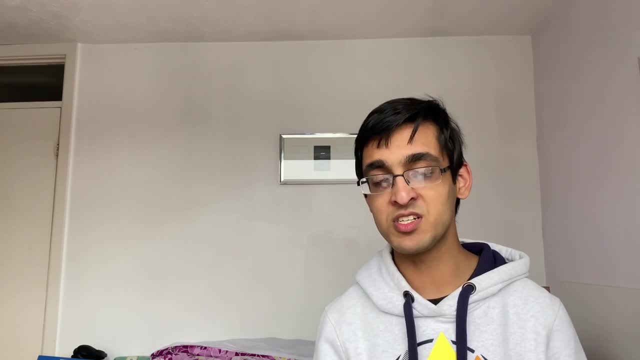 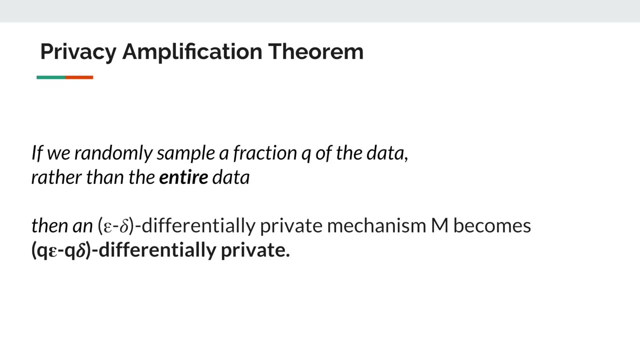 greatly. Another technique to add randomness and just preserve our privacy is to use sampling. So rather than looking at the entire dataset, you sample a fraction Q. The privacy amplification theorem says that what was previously an Epsilon Delta, differentially private algorithm. 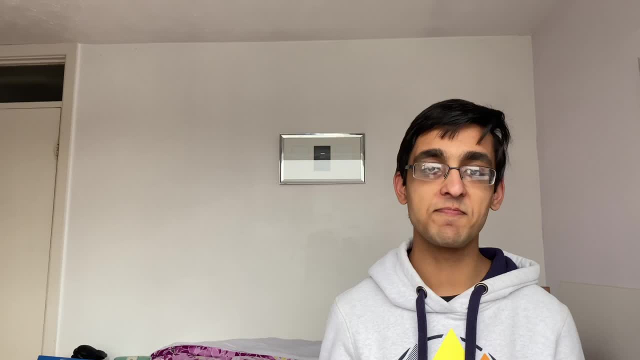 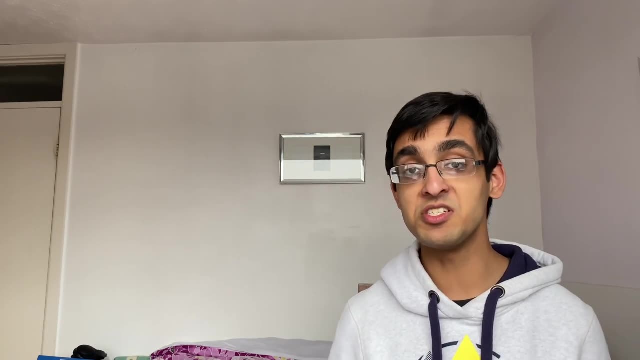 is now Q, Epsilon, Q, Delta, differentially private. Now, if you've ever played the game 20 questions, you'll know that by asking enough questions, regardless of noise, you can hone in on the correct answer, And the fundamental law of information recovery says that privacy can. 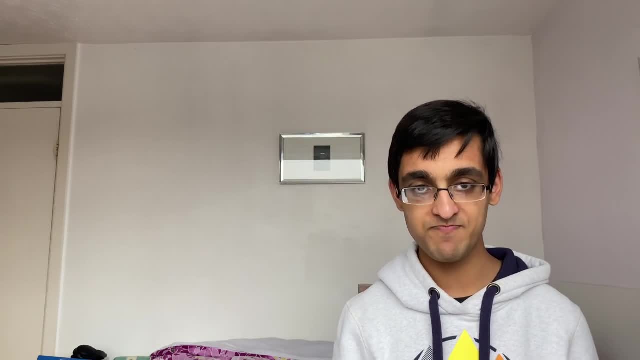 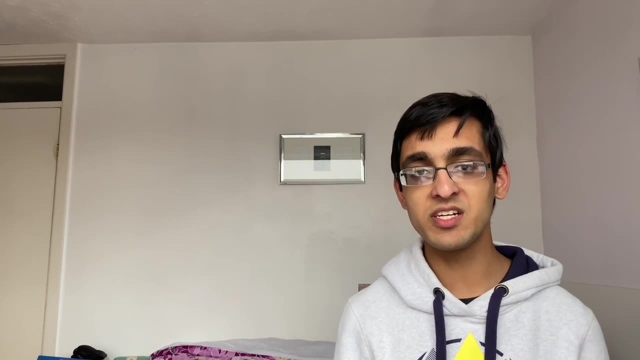 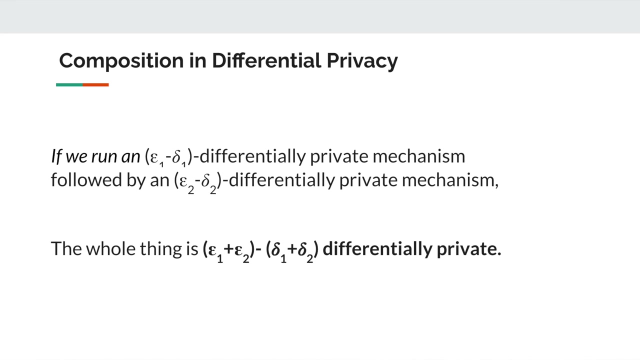 just be eroded by asking enough overly accurate questions. So the more queries you have, the larger the privacy loss. And we can actually represent this in differential privacy quite nicely, because if we have a privacy budget of Epsilon one in the first algorithm and a privacy budget of Epsilon two for the second, 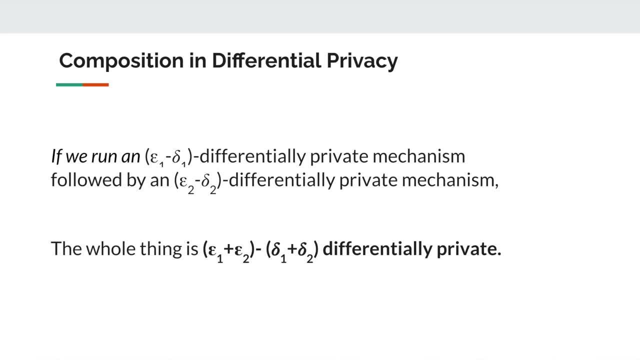 algorithm. if we run them together, then the total privacy budget that we need is less than or equal to Epsilon one plus Epsilon two, And so there's this really nice composition property of differential privacy. So we can analyze each of our subroutines in turn and then just add up the privacy budgets. 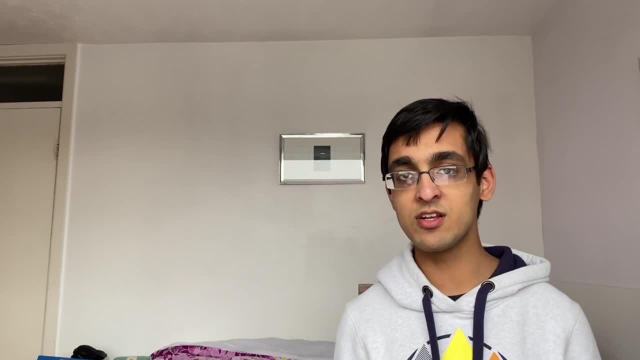 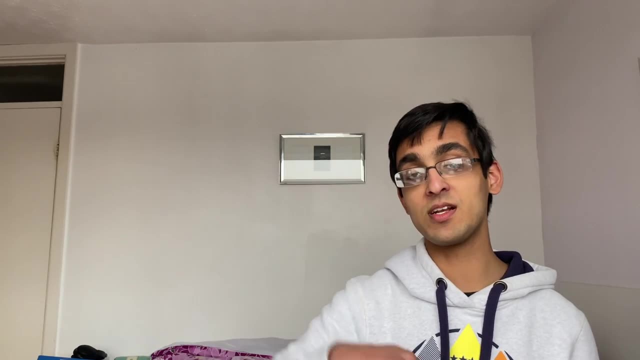 to figure out the total privacy budget required. So I want to switch tack now and look at the seminal paper that applies differential privacy to deep learning. If you're finding this video useful, please drop a like. This paper modifies stochastic gradient descent to become differentially private And 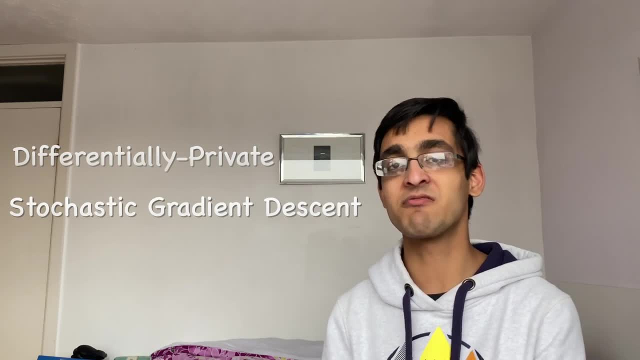 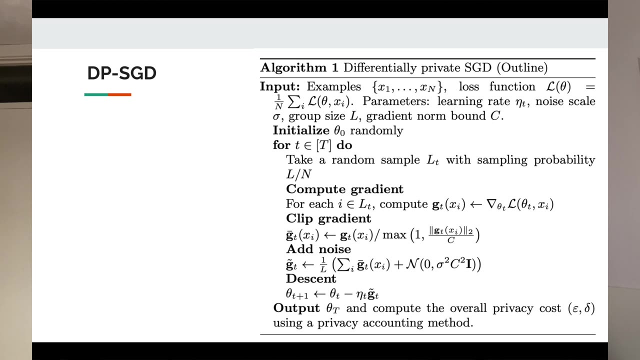 the algorithm is known as differentially private stochastic gradient descent, or DPSGD for short. The aim of the algorithm is to limit the privacy loss per gradient update. So rather than updating with the raw gradient, we first clip the gradient so it has a maximum gradient norm of C. 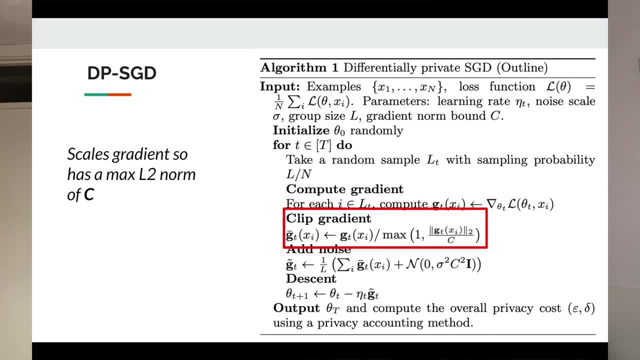 And this intuitively limits the amount of information that we're learning from any given example. And then we add our noise, So we sample from our Gaussian distribution standard deviation of C, Sigma, And we can tune these hyperparameters, C and Sigma, to give us our 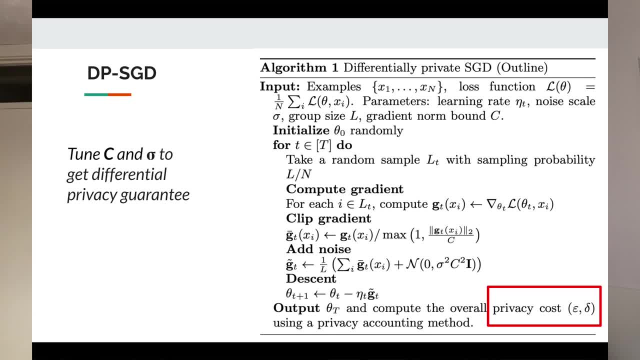 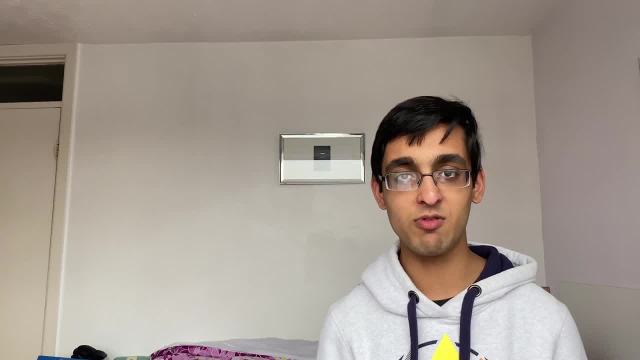 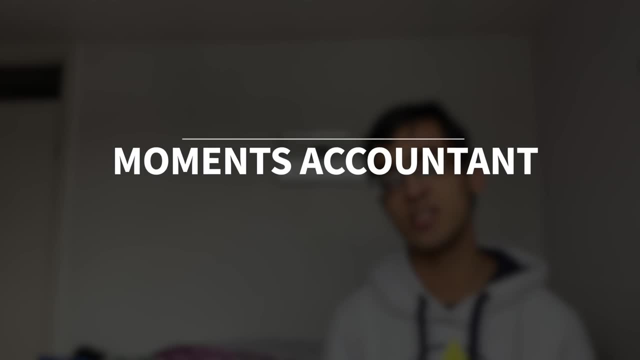 particular Epsilon delta guarantees for each step of gradient descent. So this looks like an individual step of gradient descent, But what about the overall privacy budget required? This is where the second, third contribution of the paper comes in: the moments accountant technique that we use to track our 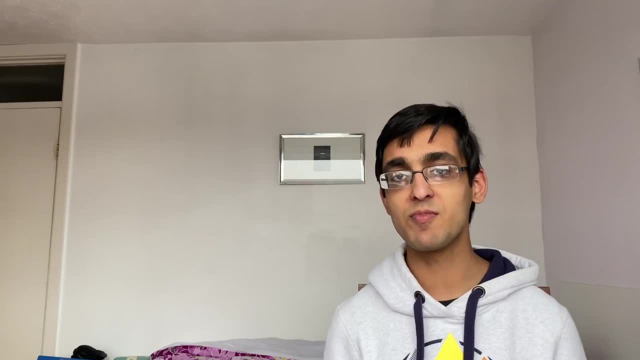 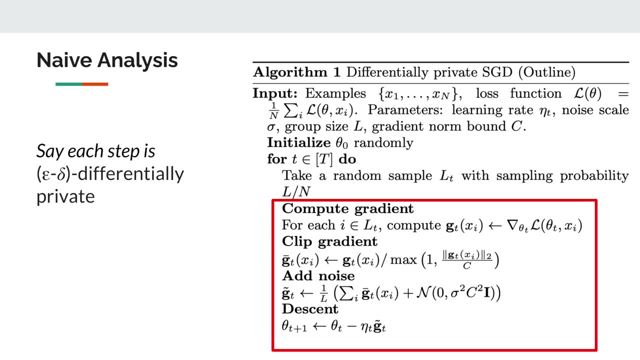 privacy budget. So first let's look at a naive way of adding up our privacy budget. We know that each step is Epsilon delta, but that we're sampling a mini batch with some probability Q. So by the privacy amplification theorem, each step is actually Q Epsilon, Q delta differentially. 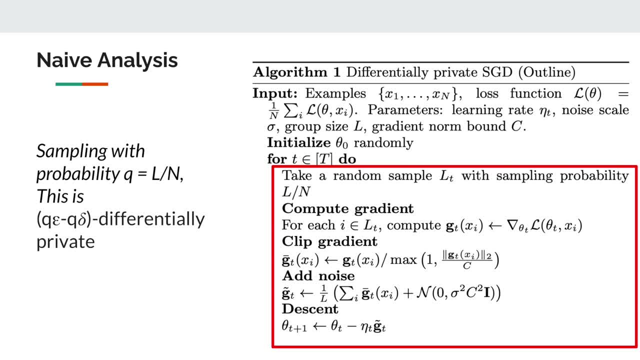 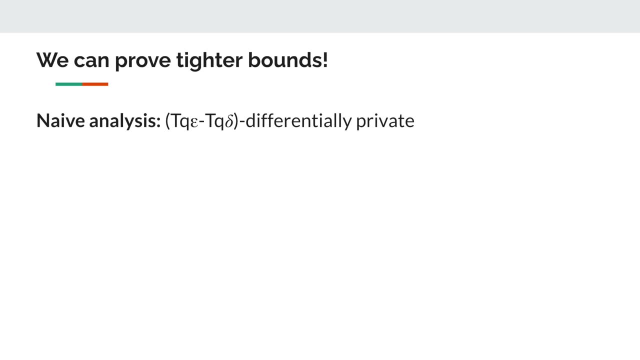 private. And if we're doing this for T epochs, we can add these all together to find that the, the overall algorithm is Q, Epsilon T, Q, delta T, differentially private. But this is actually quite a loose upper bound And actually there's a strong composition theorem. 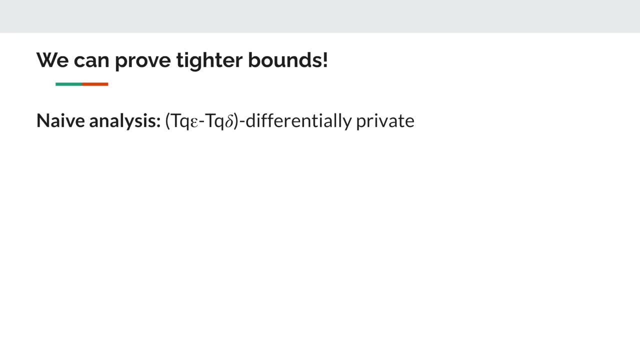 that states that you can get a tighter bound of order: Q Epsilon, root T, log one over delta and T Q delta. So we've actually improved on our budget. So actually, rather than it being proportional to T, now it's proportional to root T, so you can run it for a longer number of epochs, But we can go. 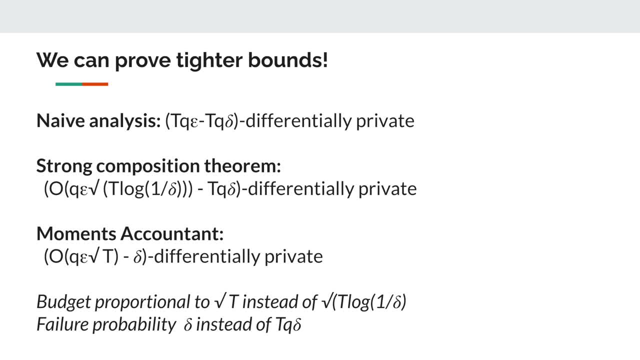 even better. And this moments accountant technique that the paper proposes actually gets the bound down to order Q, Epsilon root T. So you're saving that factor of log one over delta And the failure probability is no longer T, Q, delta, but just delta. Now the maths behind the moments accountant. 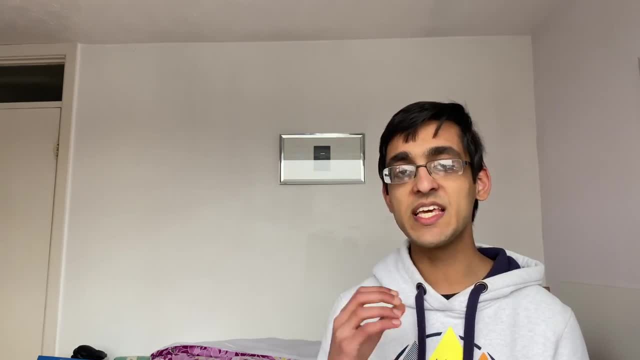 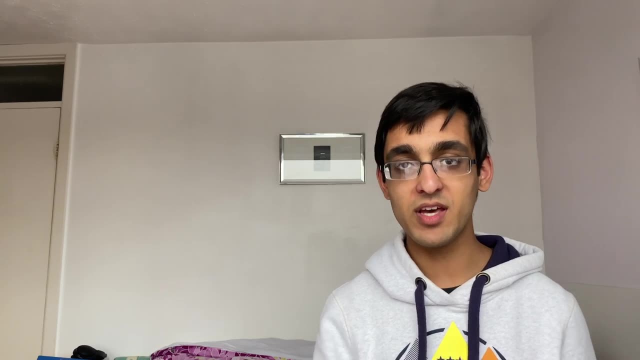 technique is very involved, So I want to give you a high level intuition. The key inside the math that authors had was that this privacy loss that we're calculating is actually a random variable of its own And we can plot it as a distribution. This distribution has a really 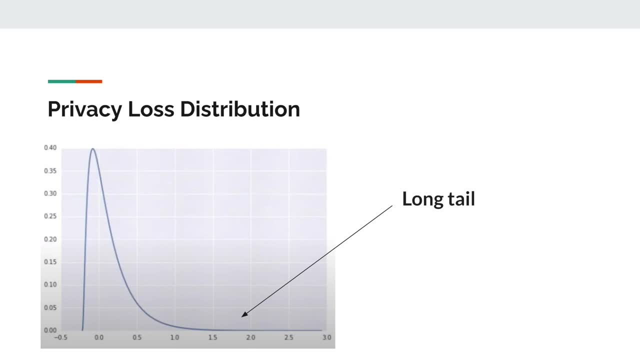 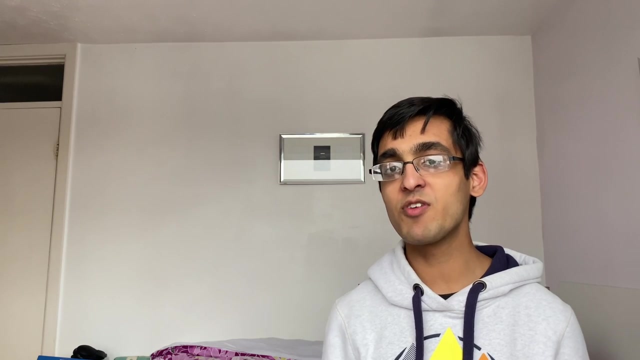 long tail And at any point we can decide to clip the privacy loss and decide that this is our privacy budget And so our failure probability. delta is actually a bound on the probability of that long tail for all the values greater than Epsilon. The reason we framed it this way as a 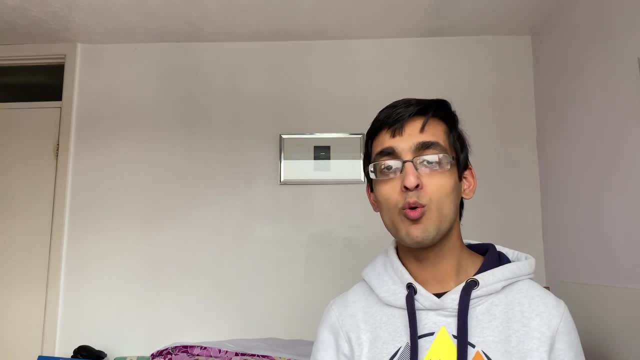 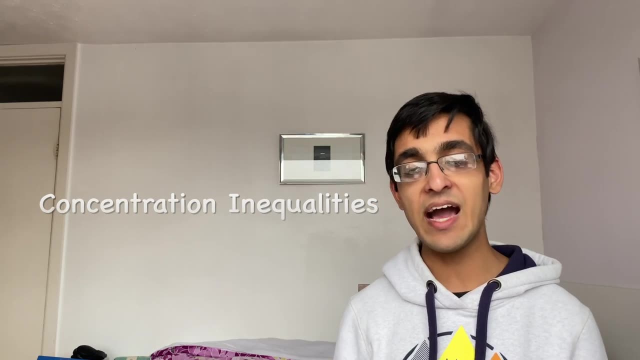 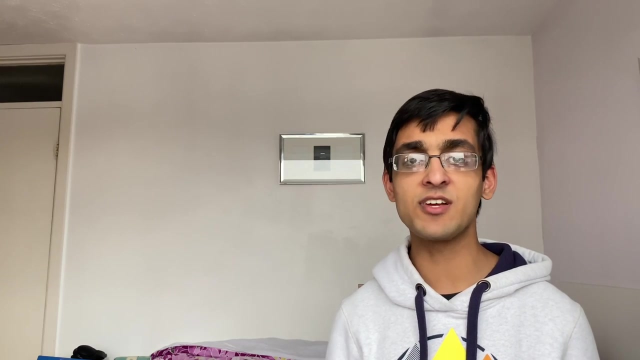 probability distribution is that now we can apply all our theorems of our probability distributions to this, In particular concentration inequalities, which look at how the probabilities vary as you go away from the mean distribution. So we know for a Gaussian distribution that 95% of the values lie within 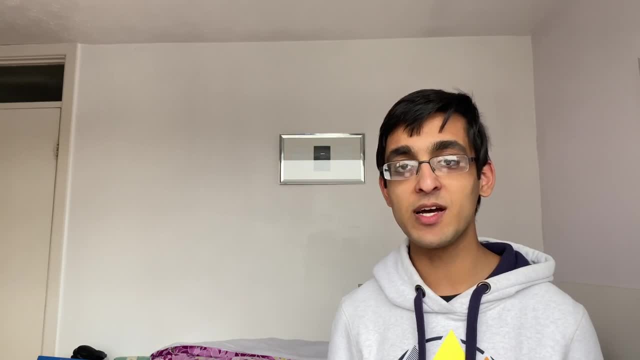 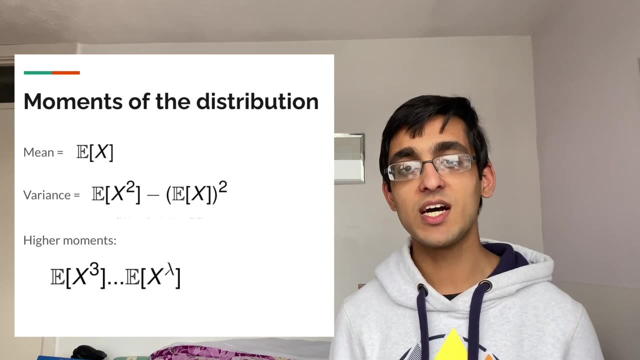 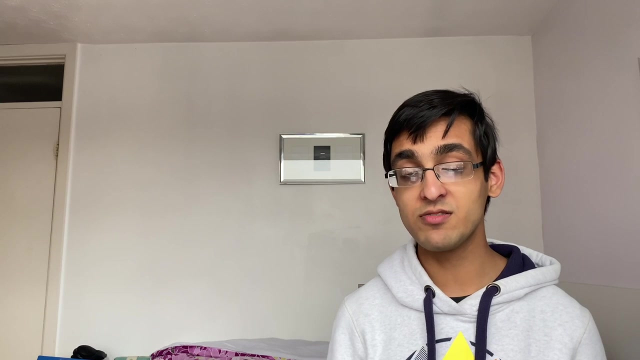 two standard deviations of the mean. So we can get tighter bounds by looking beyond the mean, which is the expectation of this distribution, X And the variance, and look at higher moments, So the expectation of the variable X to the lambda. And so what the moment accountant does is throughout training it keeps track of all. 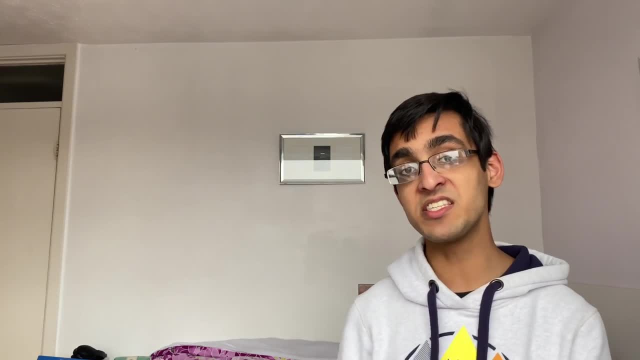 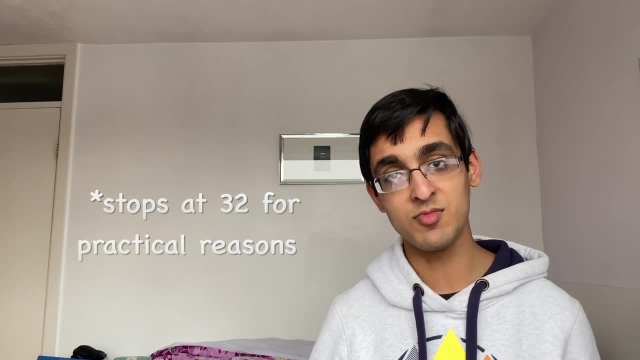 these bounds associated with each of the moments and then picks the tightest bound. So it will choose from the first moment, your mean all the way up to the 32nd moment, And so if we look at the graph of the results from the paper, you can see that this moment accountants technique. 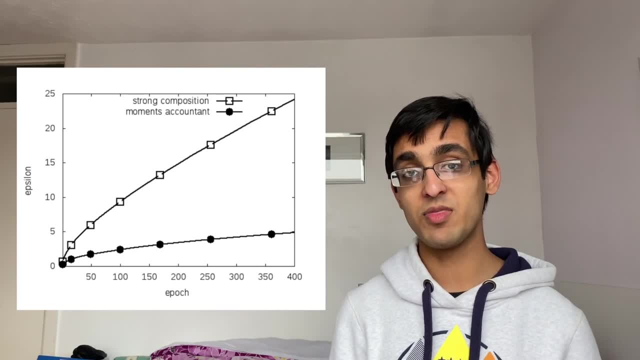 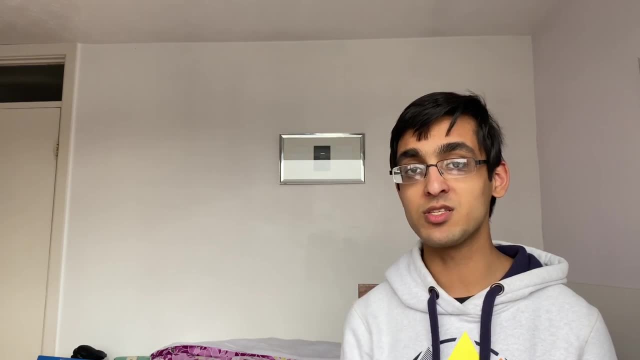 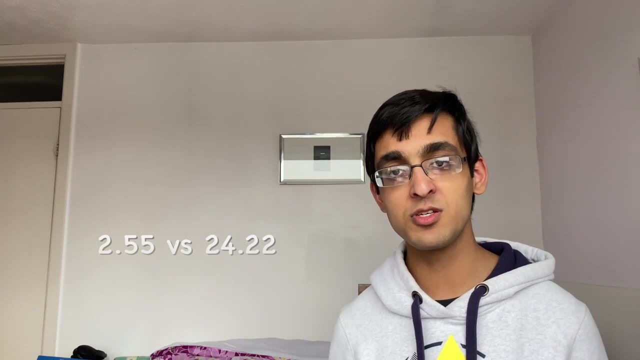 vastly outperforms the strong composition theorem. And for the same problem, they found that the moments accountant technique found that we need a budget of 2.55, versus the previous guarantees which would only bound it to 24.22.. And having a tighter upper bound on our privacy. 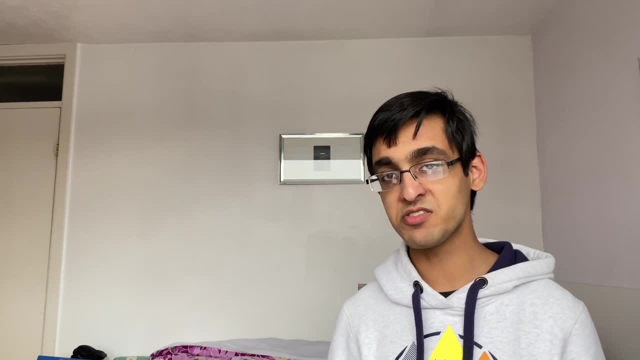 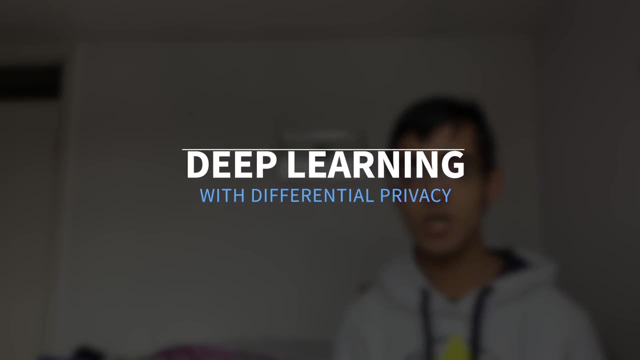 budget means that we're no longer overestimating the privacy loss of our algorithm as much, And so we can decide to reduce the noise or run our algorithm for longer. Okay, so how do we use differential privacy in practice? Well, it turns out it's just a case. 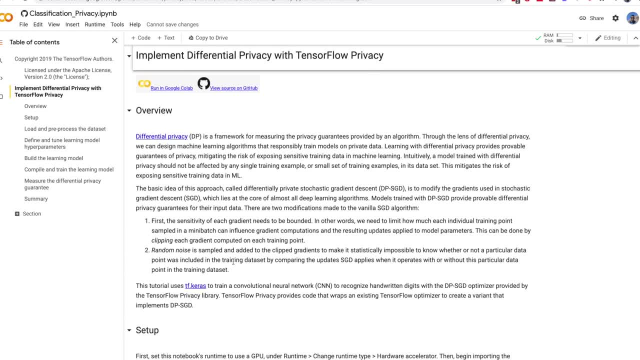 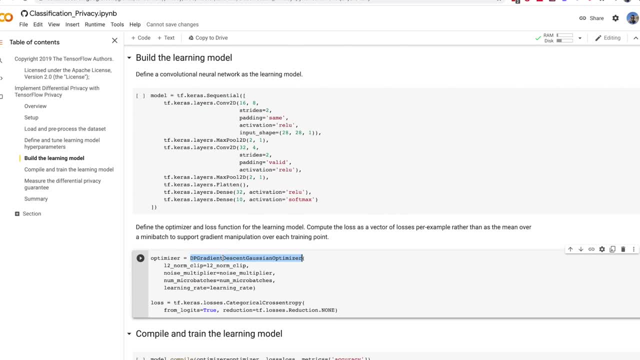 of swapping your standard optimizer in your neural network with a differentially private one. DPS-GD is actually implemented for us in the TensorFlow privacy library And they have an example Google Colab notebook which I have linked down in the description below. So this optimizer, as you can, 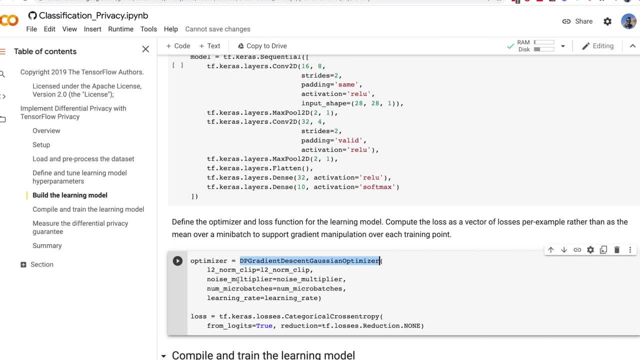 see, takes in a hyperparameters for the noise multiplier sigma and the gradient norm C, But it also takes in a third hyperparameter, the micro-batch size. This is an implementation detail designed to make the algorithm run faster Rather than clipping each gradient individually. 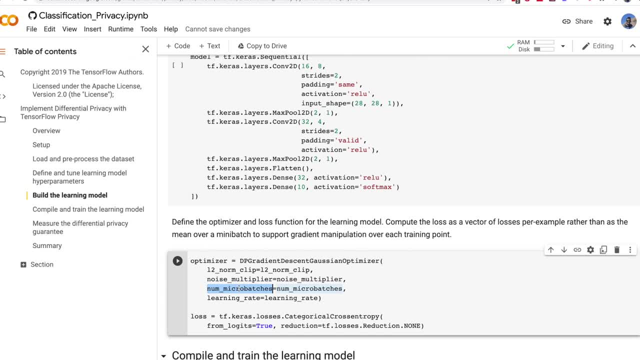 we can average the norms over a micro-batch, So say of 32 examples in your overall mini batch of 256.. Now with DPS-GD, we no longer need to do learning rate decay because in practice, because of the noise of differential privacy, we never get to a point where we need to decay our learning rate. 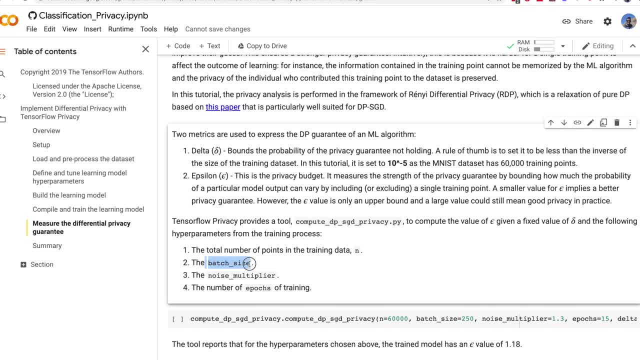 this noise can be varied by changing your mini batch size. so a smaller mini batch size will mean a more noisy update, but you get better privacy guarantees because your sample fraction is that much smaller, whereas a larger mini batch results in a less noisy update but less privacy. 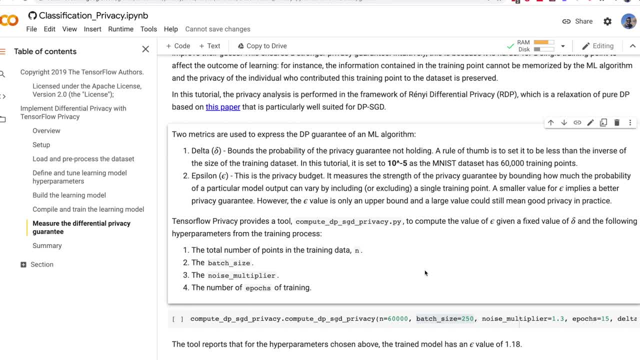 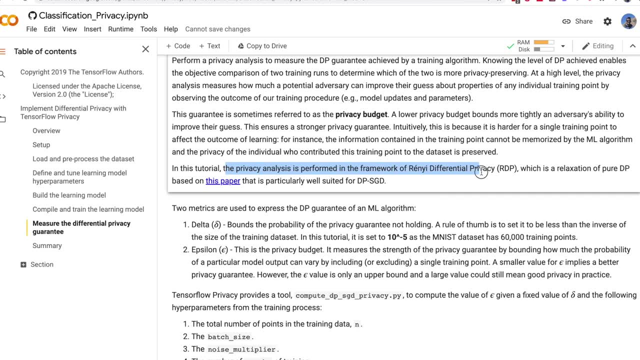 pyTorch also has a library for differential privacy called obocus, and both the tensorflow library and the pyTorch library actually use a slightly relaxed form of differential privacy called ren-y differential privacy, which we'll cover in a future video below. so be sure to. 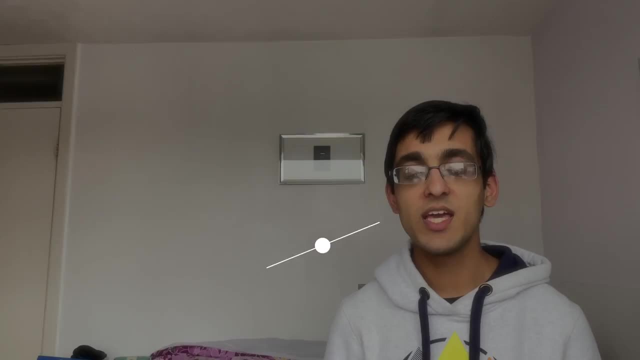 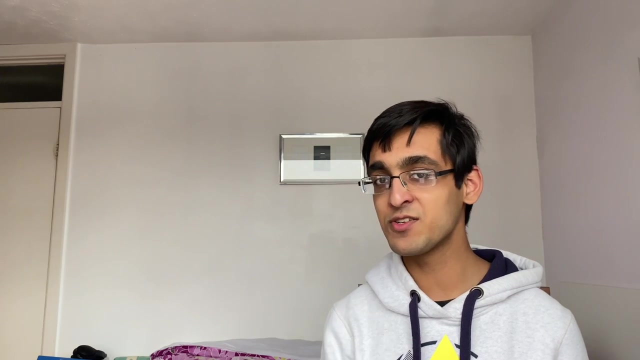 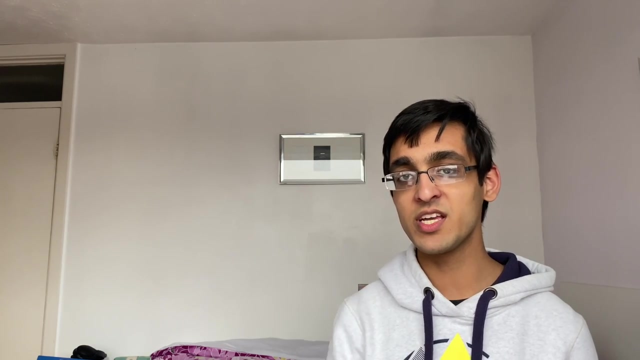 subscribe. DPS-GD isn't perfect. in practice this only works for large data sets where the privacy loss on each individual example is that much smaller because of the size of the data set, but it results in less privacy gains over time the size of the data set, so you don't need as much noise to train the model. 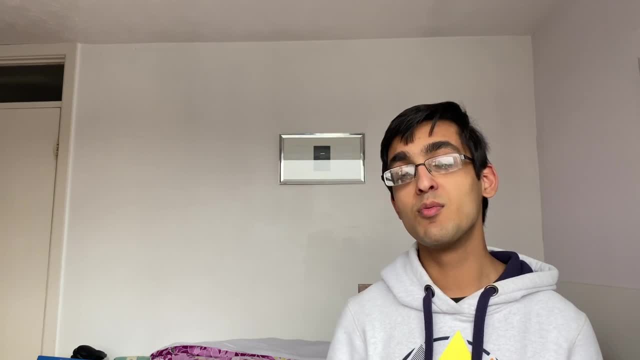 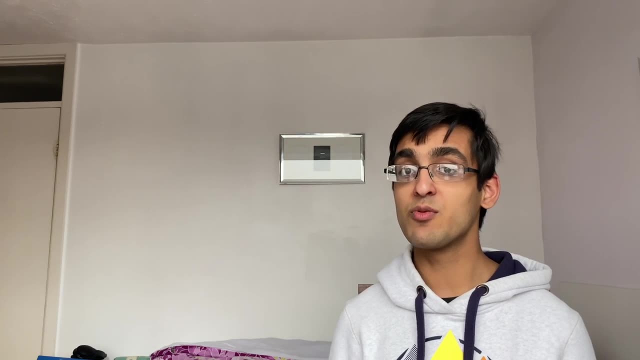 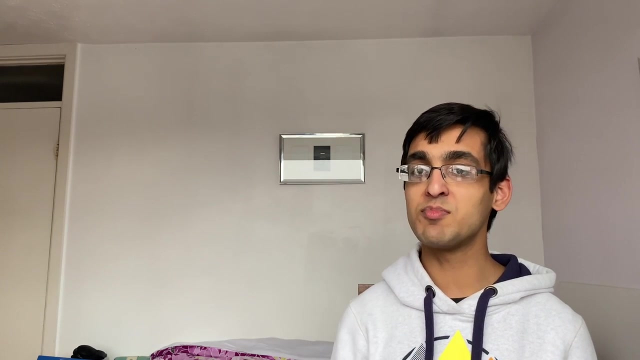 The noise also affects minority subgroups more than majority subgroups, so differential privacy actually has an impact on fairness, which we'll also look in a future video in this channel. And finally, DPSGD is just one way of training a deep neural network with differential privacy. In a future video. 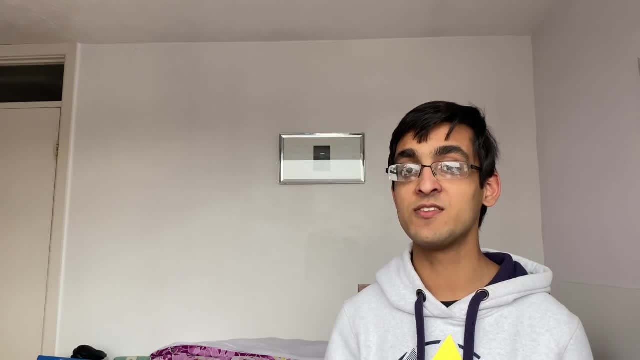 we're going to be looking at PATE, another way of ensuring privacy in your model. So be sure to subscribe and hit that notification bell to be notified when I release the next video.